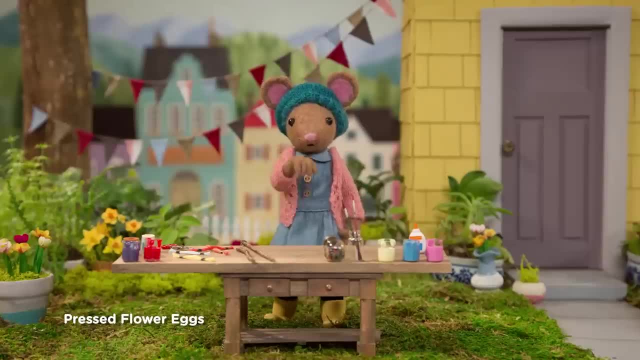 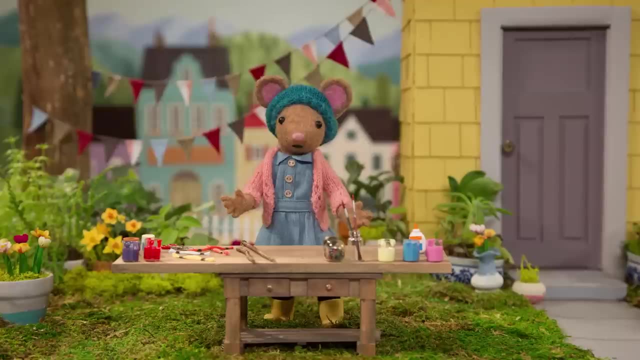 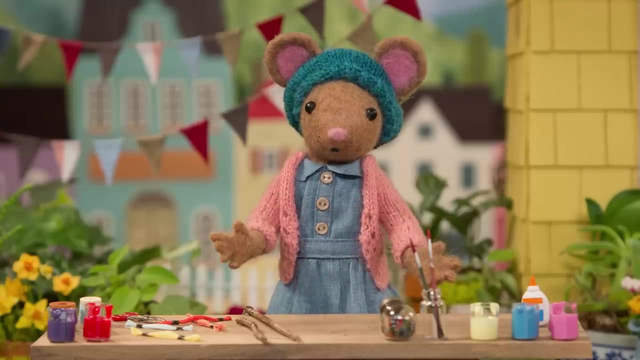 Hello Gumboot Kids, Hi Daisy, It's springtime, my favorite time of year. Flowers are in bloom again and the signs of spring are everywhere. It's so inspiring. Would you like to make a pressed flower egg with me? Gumboot Kids. 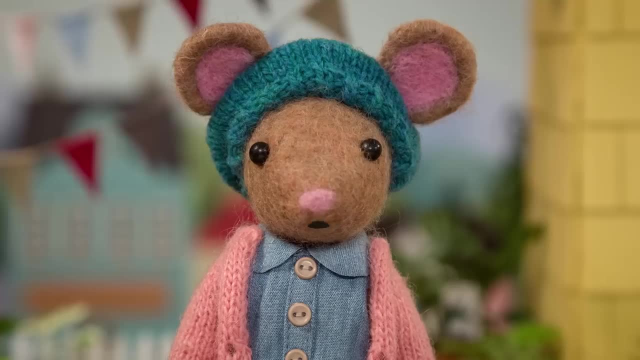 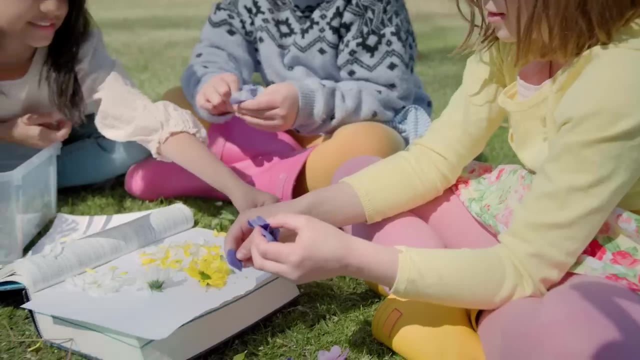 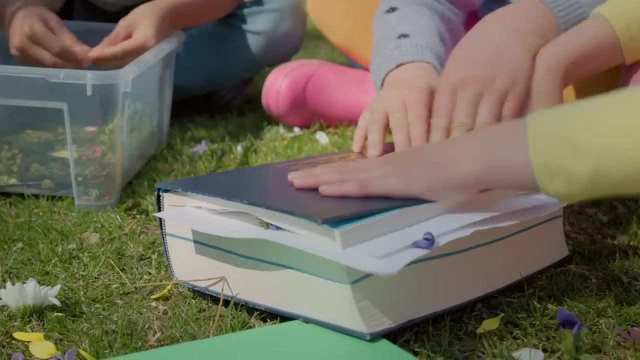 Yay, Okay, here we go. Step one: let's press some flowers, Pick some tiny flowers or pluck petals from a flower. Place them between two sheets of paper inside a large, heavy book. It will take a few weeks for the flowers to dry out completely. 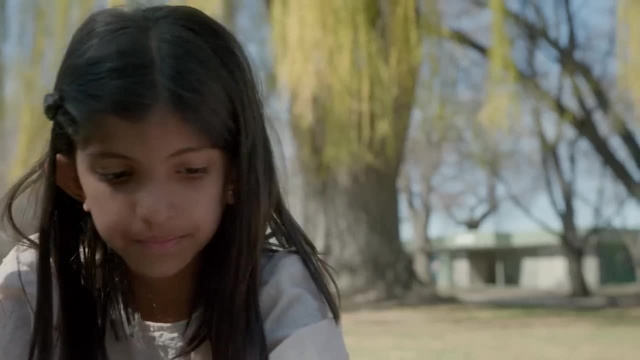 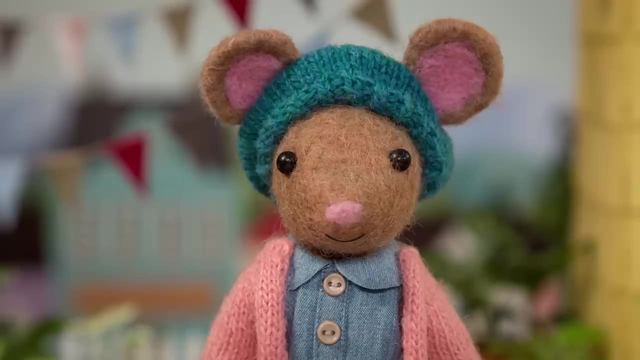 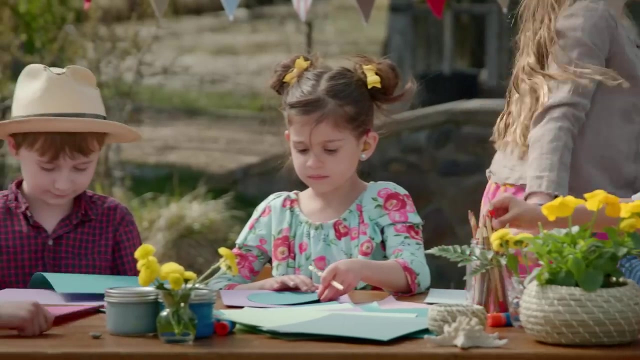 so you'll need to be patient and prepare this in advance. I love all the pretty colors- Me too. Terrific. Now step two: trace an egg shape on a piece of colored paper Like this. That's it. That's it. 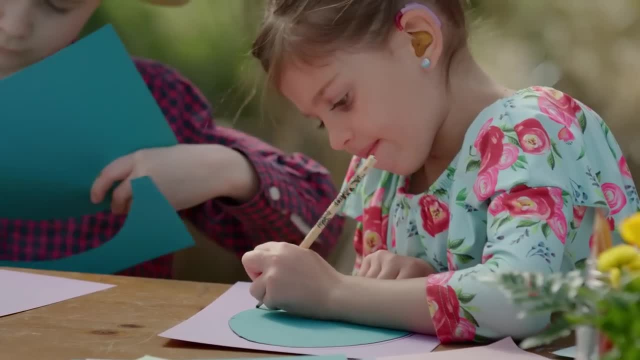 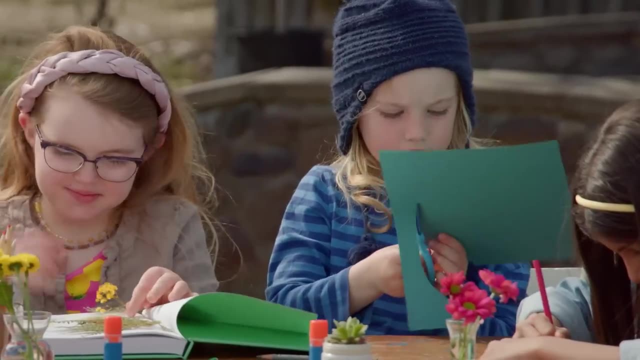 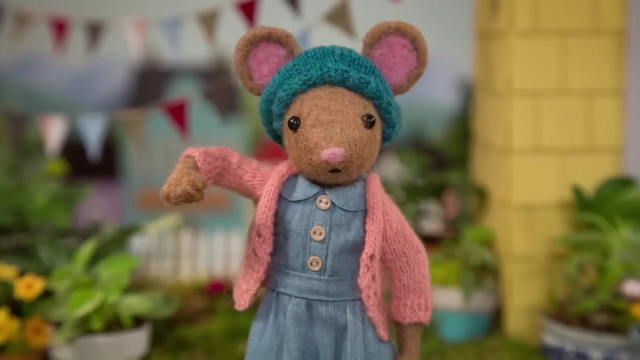 That's it, Good job. Once you've traced your egg, cut it out. You may need to ask an older friend or grownup to help you with your scissors. I can cut it out myself. Nice egg, Thank you. Great teamwork. Gumboot Kids. 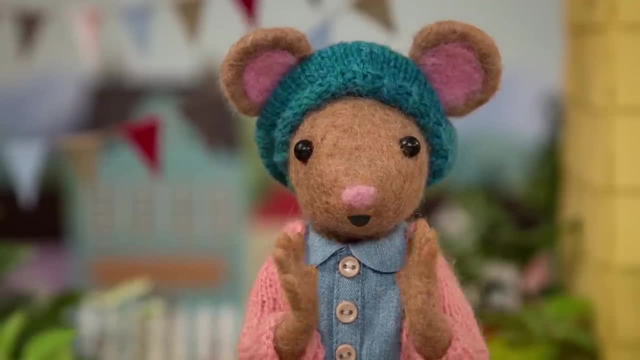 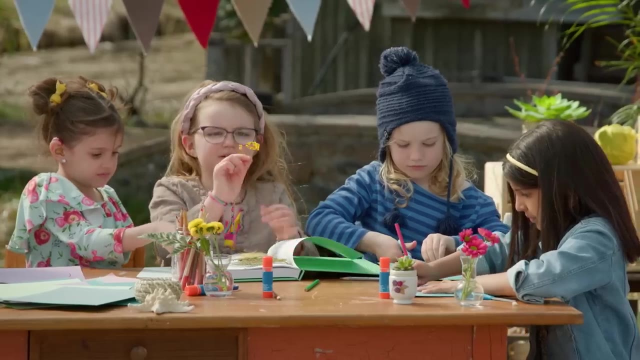 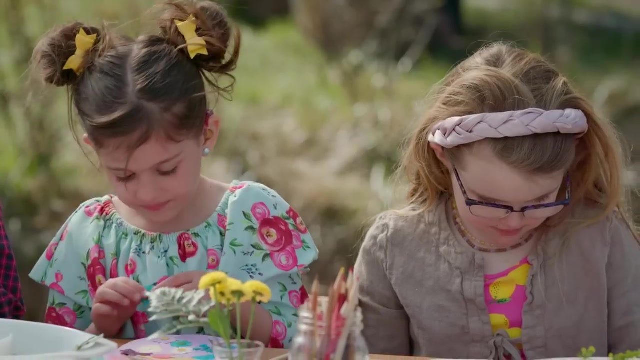 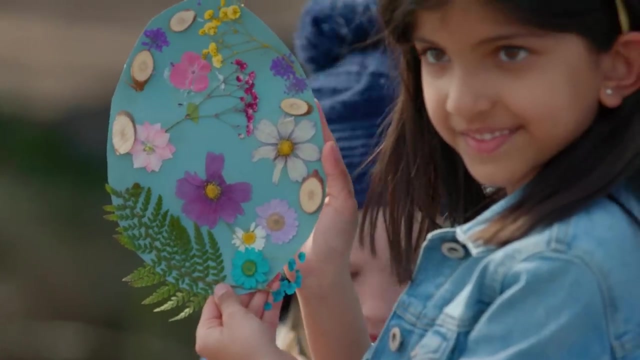 Now step three, And this is my favorite part. Look, it's our pressed flowers. How pretty. Glue your pressed flowers onto your egg. Arrange the flowers into patterns, Whatever looks beautiful to you and feels good. I like this pressed flower. 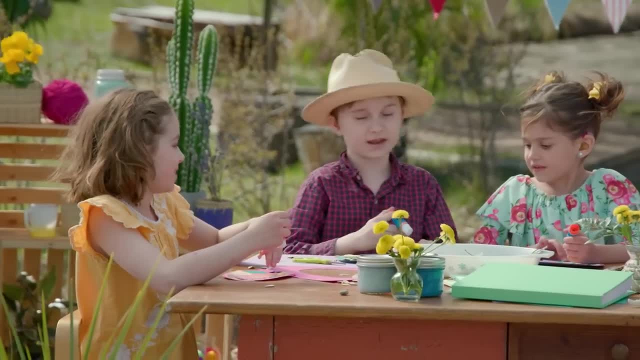 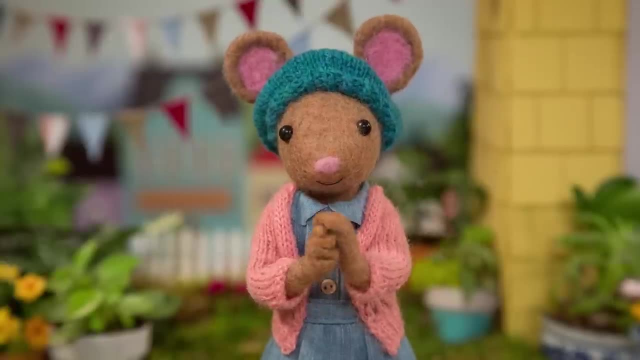 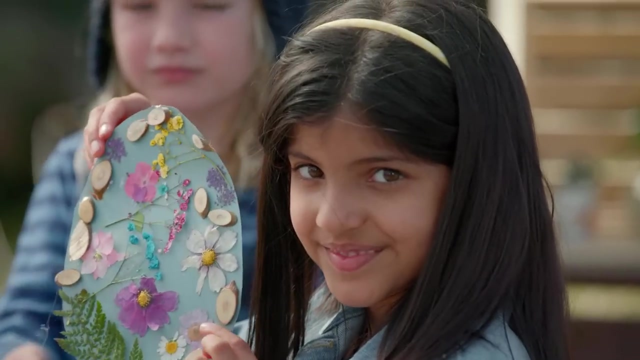 It's a hydrangea. This is so much fun. I agree, I like your egg. Thanks, The flowers are sure pretty Terrific. All right, Gumboot Kids, let's see what you've made, Oh, wow. 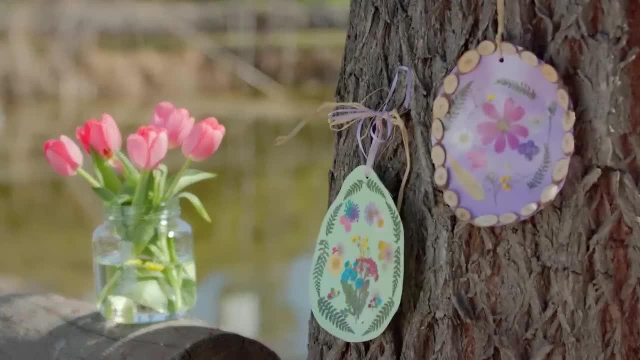 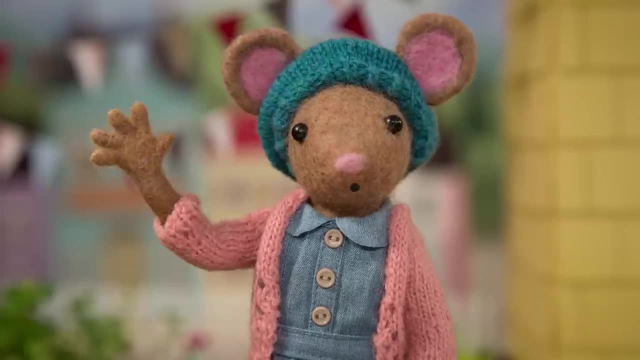 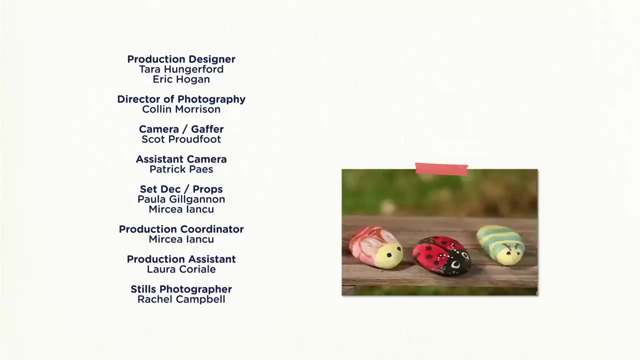 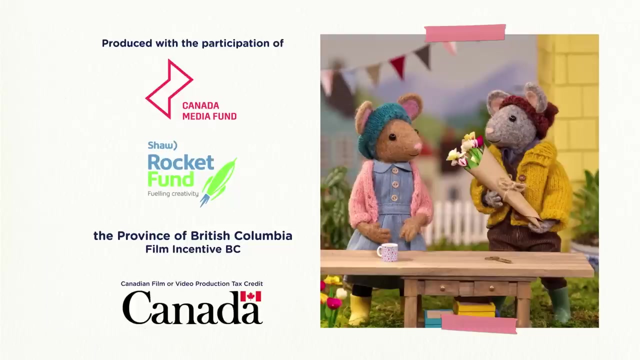 So beautiful Gumboot Kids. I'm going to hang mine and think of the springtime every time I look at it. Goodbye Gumboot Kids, Goodbye Daisy. I bet you'll make something great.